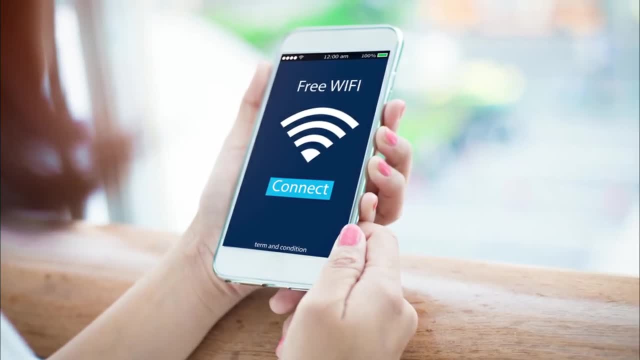 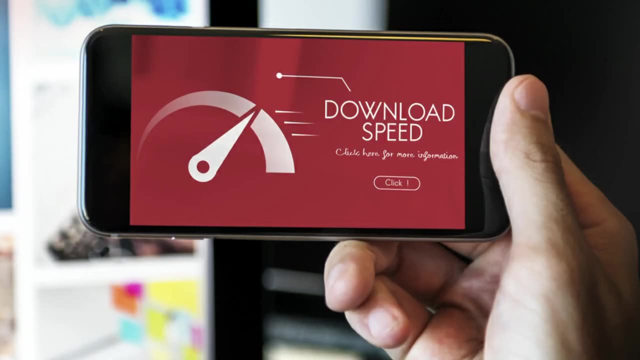 If your internet is used by your neighbors a lot and you can't say no to them, you can use this trick to limit internet speed for other Wi-Fi users except for you. By limiting their bandwidth, you will get a higher internet speed than all the Wi-Fi users. 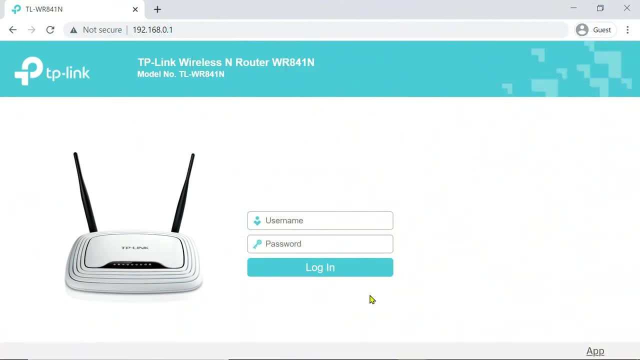 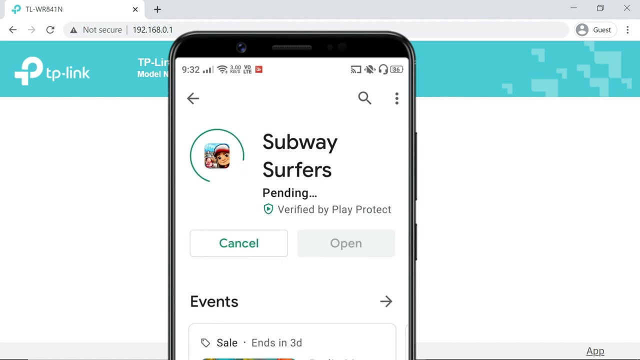 TP-Link Wi-Fi routers allow easy internet bandwidth control for all the connected devices. You can limit the bandwidth of specific devices or users that are downloading too much data and crippling the internet speed for your own use. Before limiting internet speed on a device, I want to show you my actual internet speed provided by ISP. 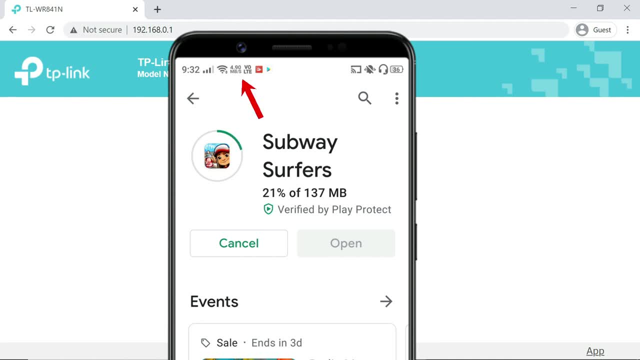 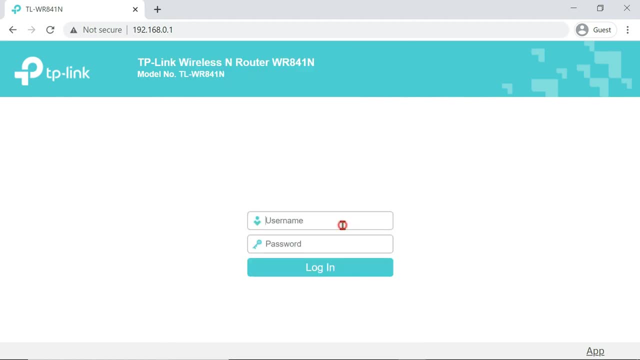 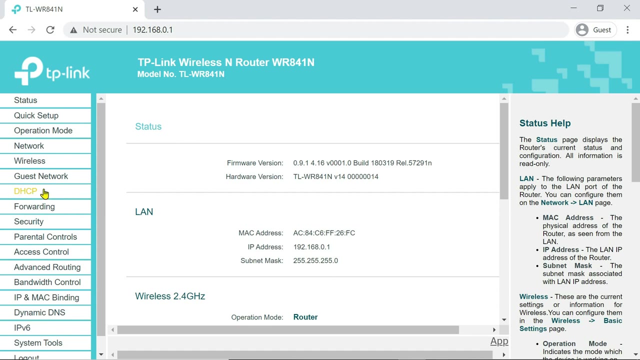 As you can see, it is downloading at 5 Mbps speed. I want to limit the bandwidth for this device to 1 Mbps. First of all, login to a TP-Link router, Click on the DHCP tab. DHCP helps to assign an IP address to your devices connected to the Wi-Fi router. 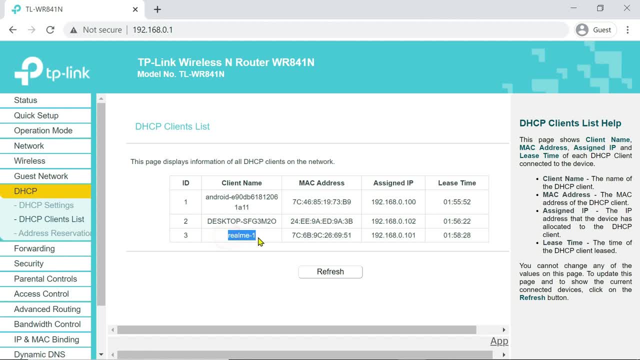 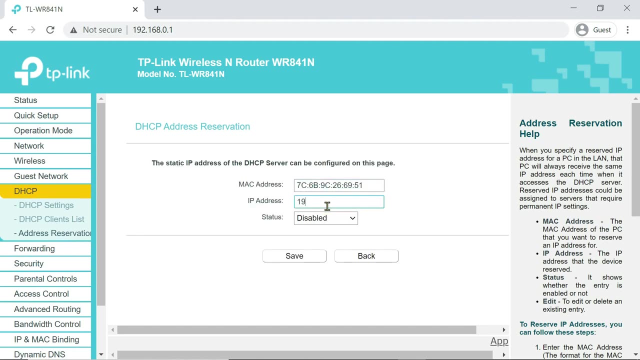 In DHCP client list you get the device name, MAC address and assigned IP address. Copy the MAC address and the IP address of the target device In address reservation. add MAC address and IP address of the device. Once you have allocated the IP address to the device's MAC address, the IP address will remain permanent for the device. 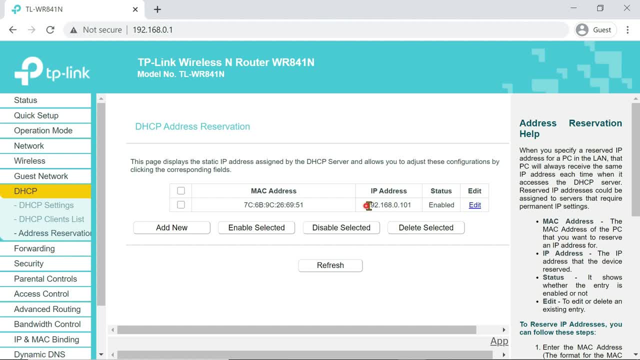 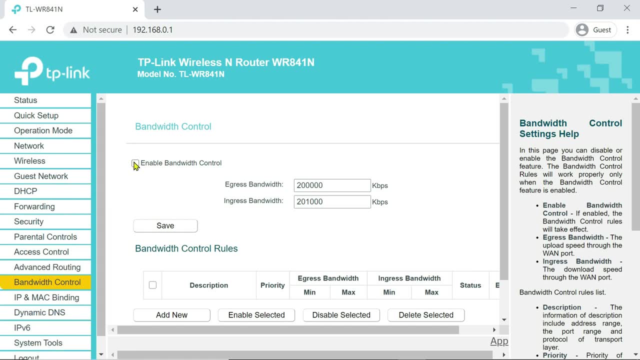 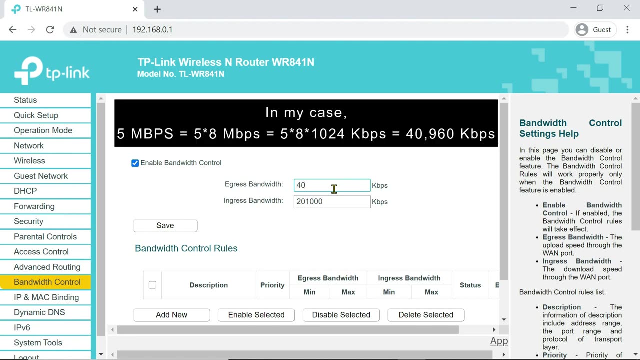 So you can easily control the bandwidth of the device using the assigned IP address. Now go to the bandwidth control. Check the box to enable bandwidth control. In the egress and ingress bandwidth field, enter the real bandwidth given by our ISP. 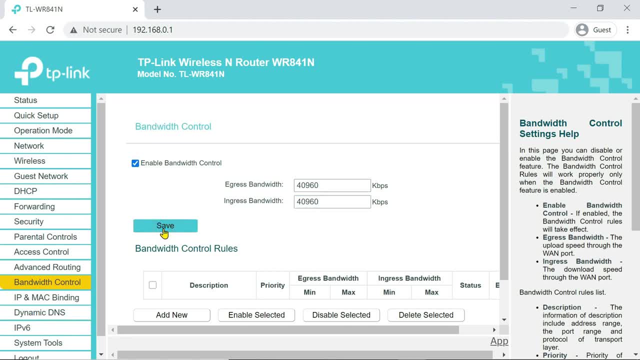 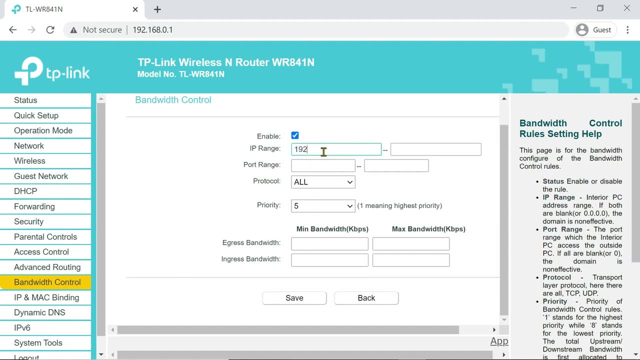 In rule setting, click add new. In IP range type: the IP you have assigned to the device In egress and ingress bandwidth field input the speed you'd like to allocate for the user. Once you're done, click on save.